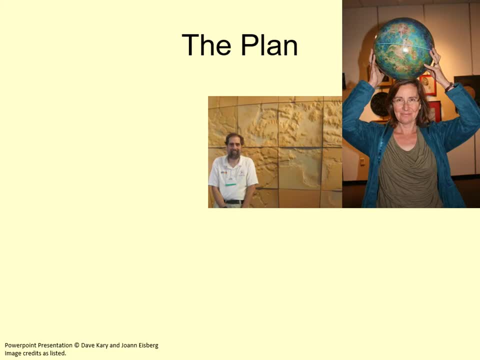 their moons. We'll start in this presentation by looking at the four important surface processes- impact, cratering, volcanism, tectonics and erosion- and a little bit of how we can learn the history of a world from studying its surface features. 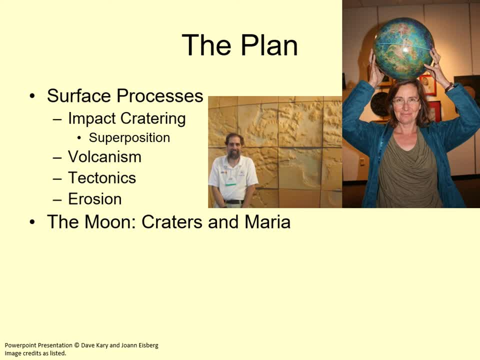 In a little bit of time we'll be talking about the four important surface processes- impact, cratering, volcanism, tectonics and erosion, and a little bit of how we can learn. The simulator files will look at examples of various planets and moons to get a sense. 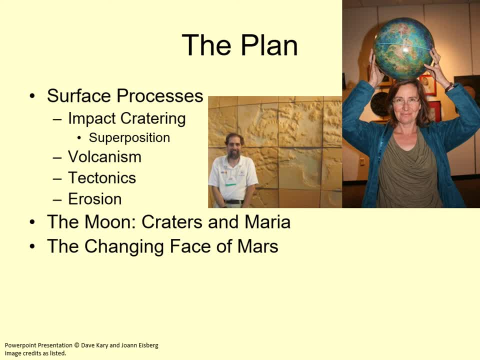 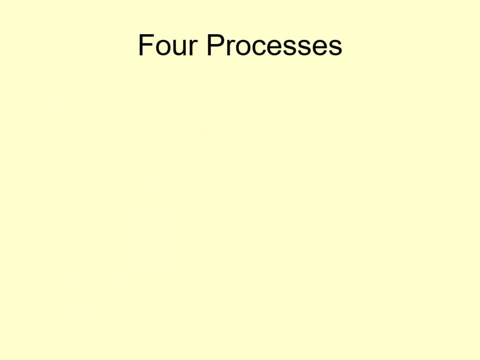 of how these surface processes interact in different ways on different worlds. We'll finish up with the Earth, the largest and most complex solid world in the solar system, and get a sense of some of the unique features of the Earth's geology. There are four major processes that shape the surfaces of solid worlds. These four processes: 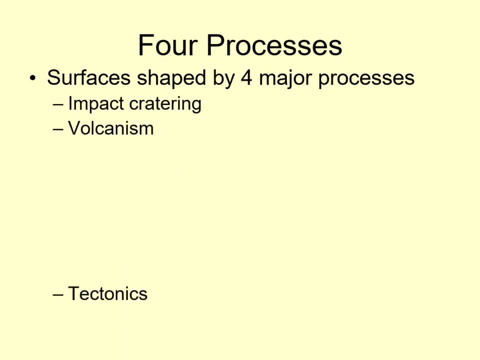 are impact cratering volcanism, tectonics and erosion. We're going to look at each of these in detail, but we should start by understanding that both volcanism and tectonics are primarily controlled by the internal heat of the planet. If the interior is hot enough that convection 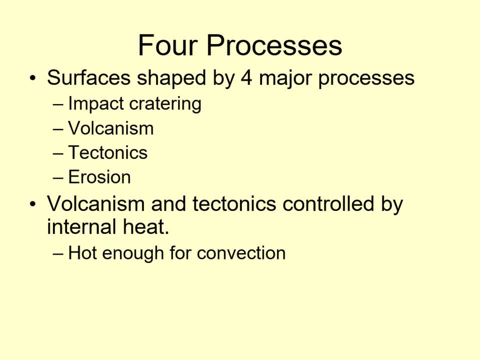 is possible inside the planet, then there will be plenty of energy to power volcanism and tectonics. Remember that this means that the interior has to be close to the surface of the planet, but not necessarily at the melting point. Composition will be important here, since 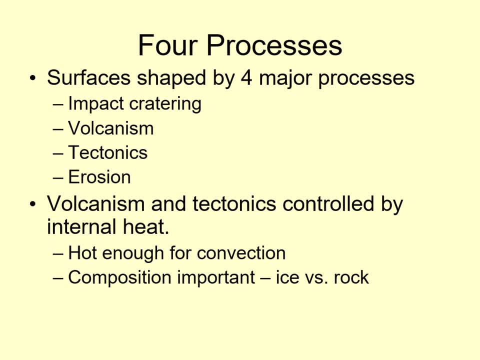 it takes a lot less energy to melt ice than it does to melt rock. Also, erosion can be related to internal heating. Erosion usually depends on having an atmosphere, and volcanism is an important way for a planet to produce an atmosphere. So what's left to shape a world? 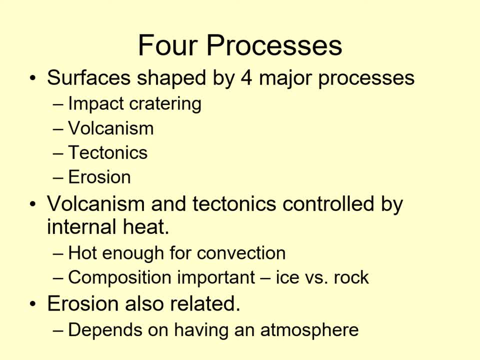 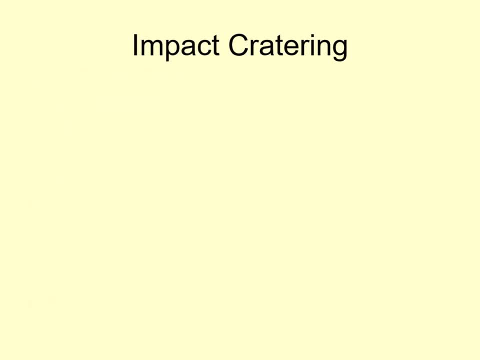 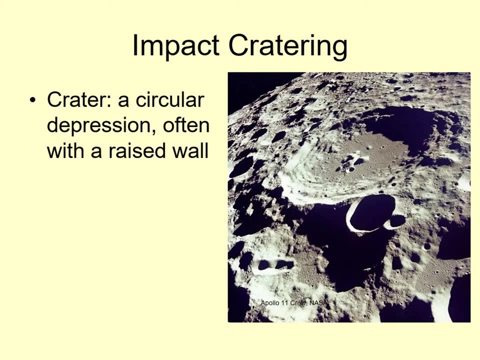 with little internal heat. Impact cratering. Impact cratering is the most important surface process in the solar system. An impact crater is a hole or depression in the ground. Craters are almost always round and they often have raised walls around the outside and sometimes other features inside them. Impact craters. 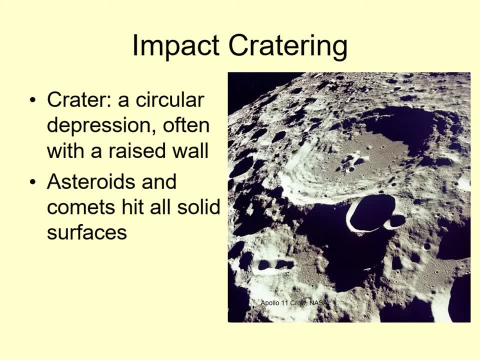 are caused by asteroids and comets hitting the surfaces of worlds. This is a good point to mention that. the crater is the hole in the ground. The crater is the hole in the surface. The impactor is the thing that hits the surface. Planets are not hit by craters. 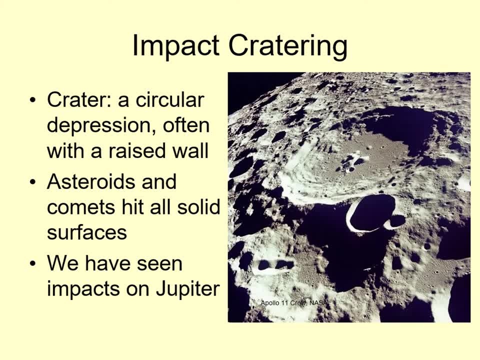 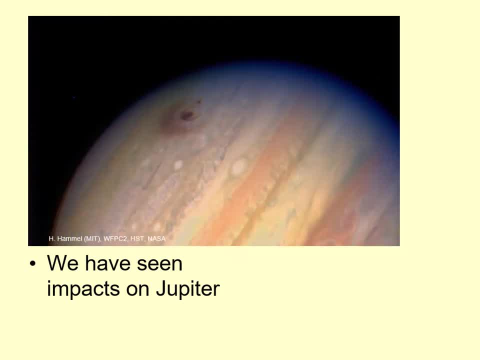 Back in 1994, we actually watched pieces of a comet hitting a planet. Unfortunately, the planet was Jupiter, so it didn't produce any craters, since there isn't a solid surface for the crater to exist on. However, it did leave black debris in Jupiter's atmosphere. 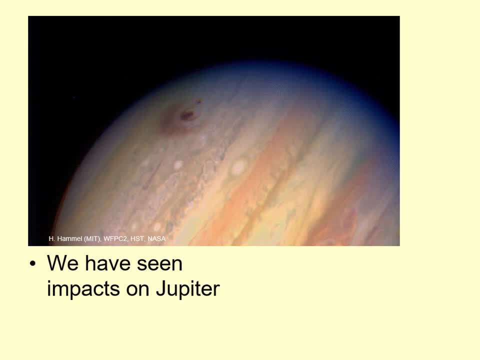 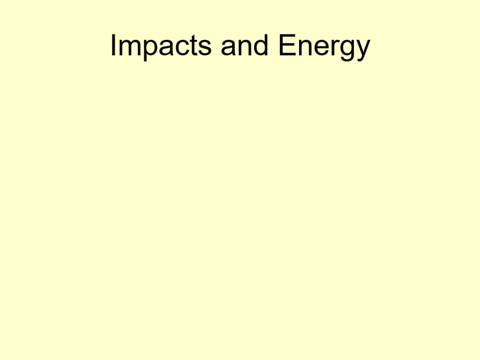 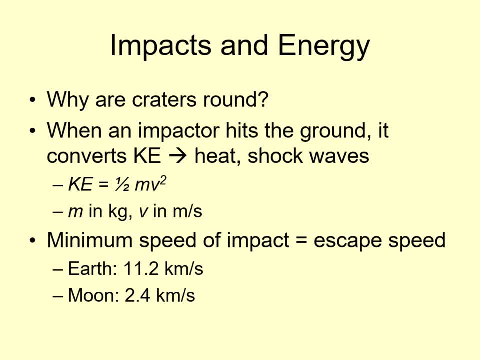 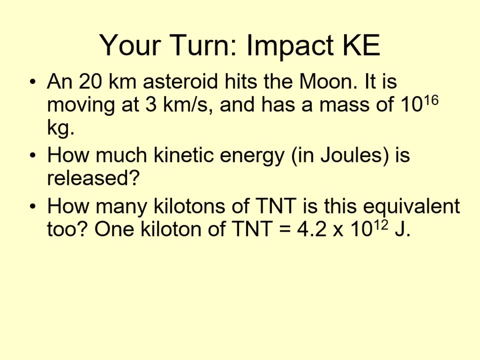 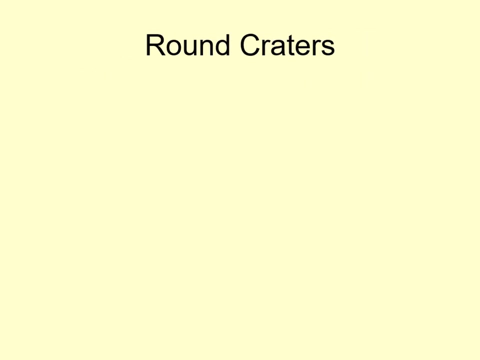 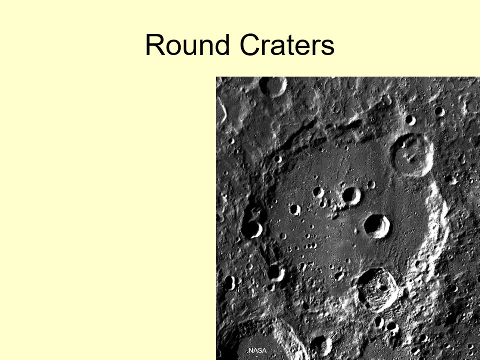 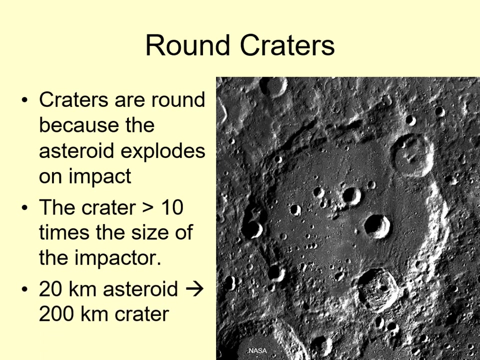 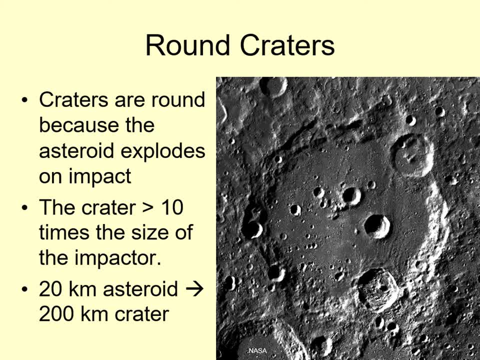 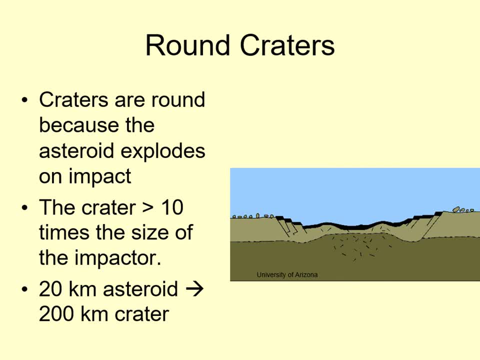 Lj us. Here is a simulation showing the steps in the formation of an impact crater. It starts with the impactor hitting the ground, Then the shock waves spread out and excavate a large region around the impactor. 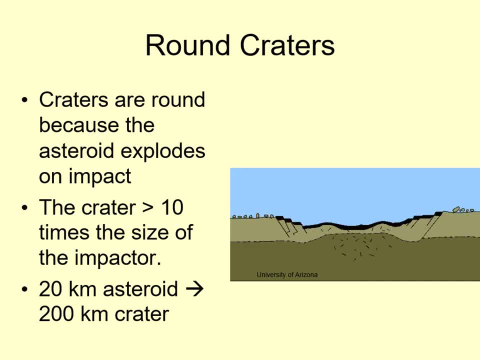 throwing material up and out of the crater as well as compressing the ground around it. In the case shown here, there is also a central peak created. Both the peak and the crater walls then slump downwards, leaving a lower peak and perhaps terraced or step-like walls. 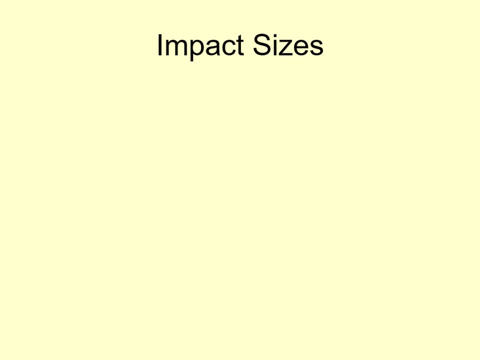 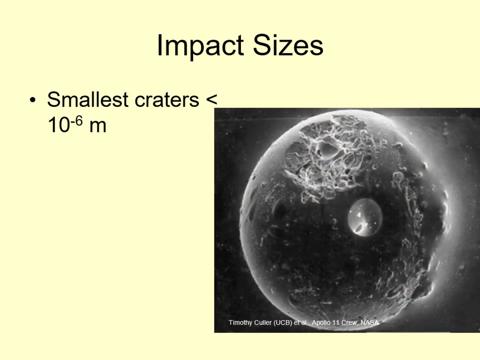 Impact craters come in a huge range of sizes. The smallest craters found are only 10 to the minus 6 meters across, smaller than the thickness of a human hair. You can see such a crater on this microscopic image of a drop of solidified lunar lava. 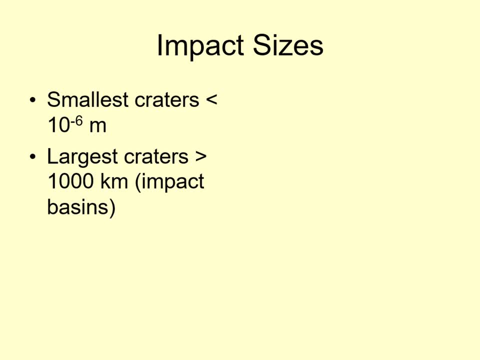 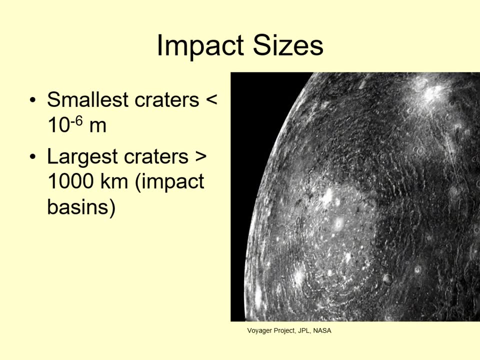 The largest craters are known as impact basins. They can be over 1,000 kilometers across, like Valhalla Basin here on the surface of Jupiter's moon Callisto. Many impact basins have multiple rings of ridges instead of just a single outer wall. 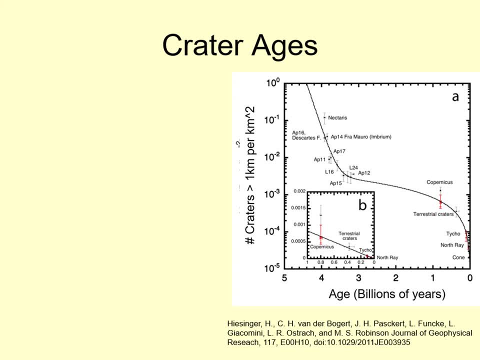 We hope you enjoyed this video. We have access to actual pieces of rock from the Earth and Moon. So on the Earth and Moon, we can use radioactive dating of rocks melted in impact to get an estimate of the ages of impact craters. Since there are a large number of preserved impact craters on the Moon, 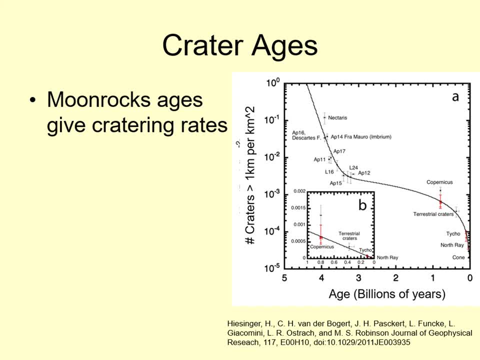 this allows us to put together an estimate of the cratering history in our part of the solar system. The chart on the right shows the result. The vast bulk of impact craters are in the solar system. Craters on the Moon formed more than 3.5 billion years ago, when the cratering rate 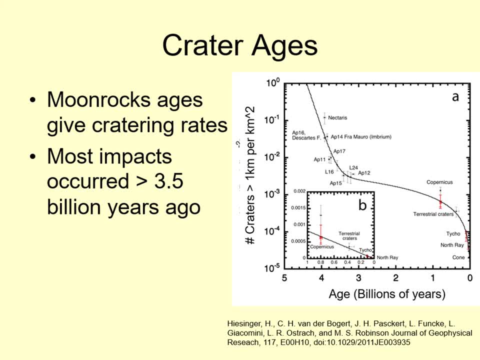 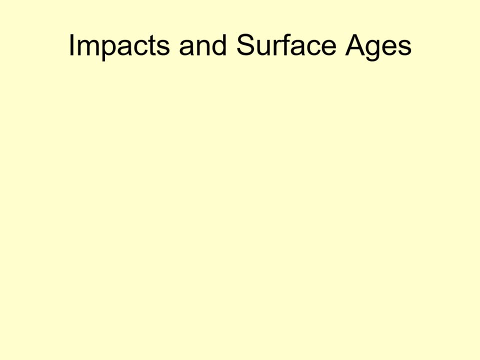 was much higher than it is today. Since about 3 billion years ago, cratering has continued, but much less frequently than in this early period On most worlds. we can't do direct measurements of crater ages the way we can for the Earth. 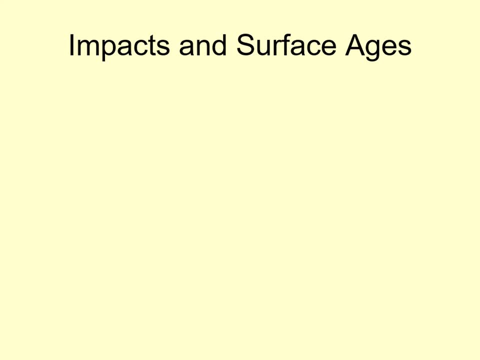 and the Moon. However, we can still use craters as a way of estimating the age of a planet. However, we can still use craters as a way of estimating the age of a planet. However, we can still use craters as a way of estimating the age of a planetary surface. 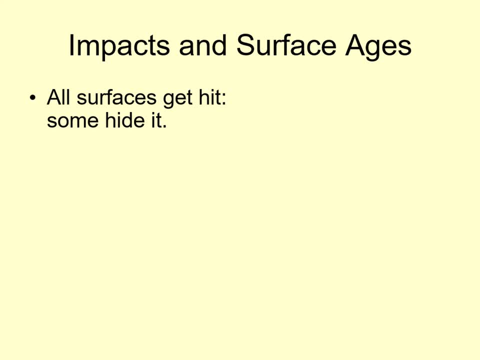 All planets get hit regularly. As we mentioned earlier, having an atmosphere like the Earth or Venus does prevent the very smallest impactors from hitting the surface, but most of the objects that produce large, obvious impact craters penetrate these atmospheres without any difficulty. 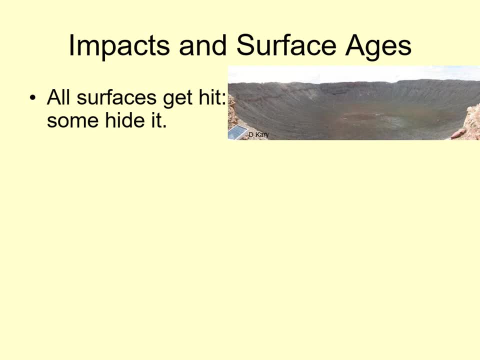 The most important thing, then that decides how many large impact craters we see on a surface is the amount of other geologic activity it has. If a world has a lot of erosion, volcanism and tectonics, then these will erase the craters. 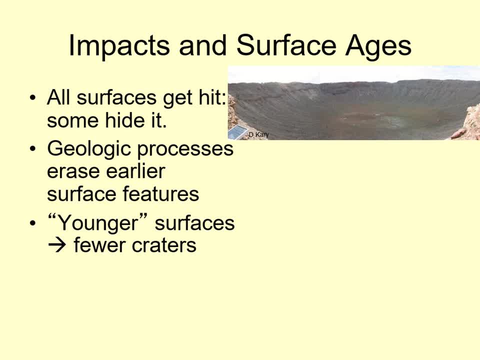 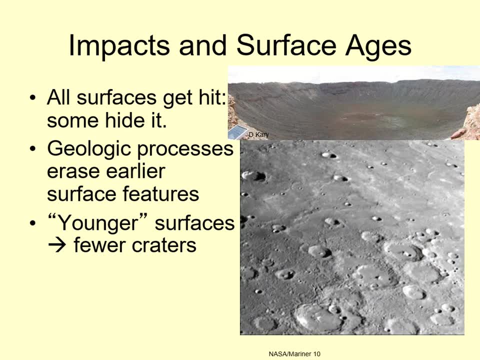 on the surface. So when we see few impact craters on the surface of a world, we describe it as a young planetary surface. In this picture of the surface of Mercury, we see there are relatively few craters in the top half of the image because lava flows have covered over all of the older impacts. 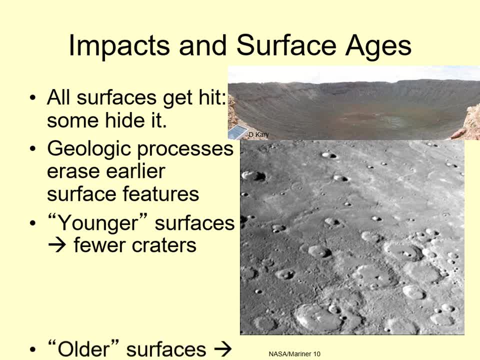 leaving just the more recent ones visible. On the other hand, if a surface has very little volcanism, erosion or tectonics, then we'll see lots of impact craters and we describe it as an older surface. In the bottom half of the picture you can see there are many more craters. 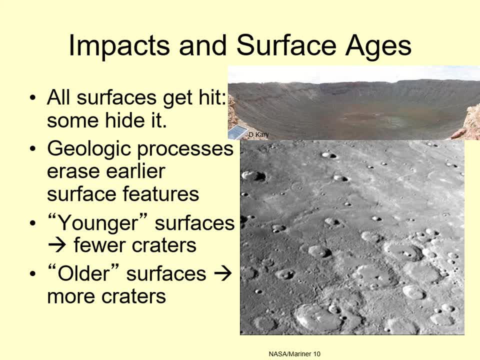 In fact, there are almost as many craters as on some of the older parts of the Moon's surface. This suggests that the older region may date back to the period almost 4 billion years ago, when the cratering rate was still very high. 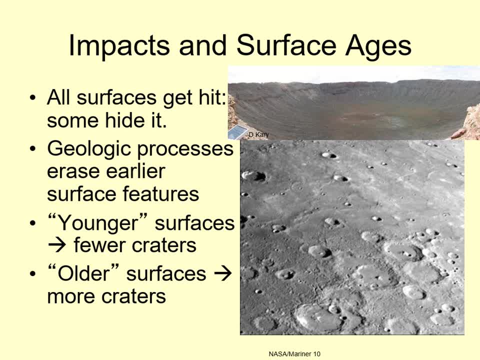 Note that when we talk about the age of a planetary surface, we're really talking about how recently the surface has been refreshed, not the age of the world as a whole. There's no reason to expect that any of the worlds in our solar system to be any younger. 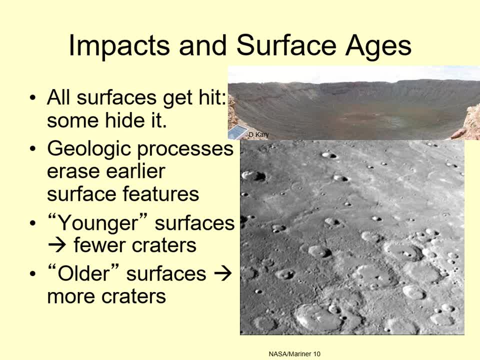 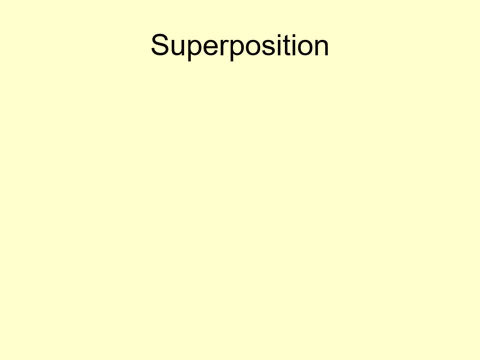 than 4 billion years old. It's just that many are good at hiding their age with some cover-up and others use a kind of peel. What we just saw regarding impact craters is really just one example Of an important geological concept called superposition. 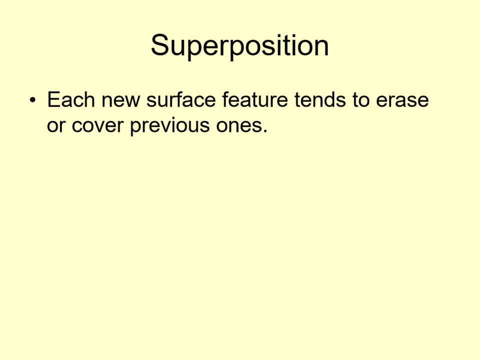 The idea behind superposition is that each time a new geologic feature forms, it tends to cover up or erase the ones that were previously there. So a volcanic flow will bury an impact crater, or the formation of a crater will destroy a river channel.